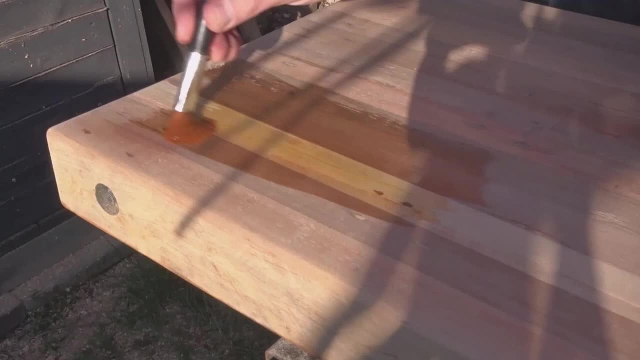 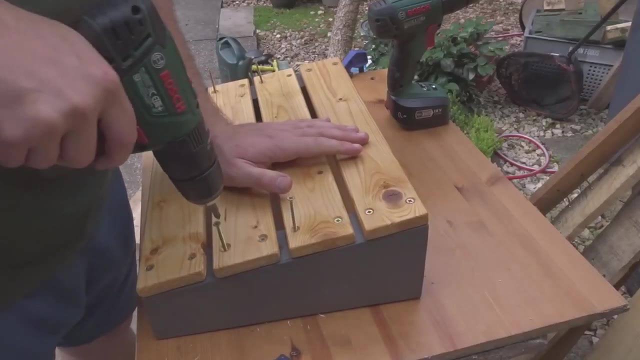 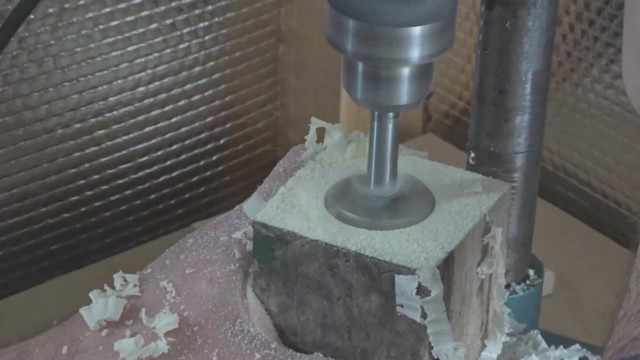 and I've put together this top 10.. This isn't just pallet wood. on this one, it's any scrap wood. If you'd like to see the full length versions of these videos, I'll leave links in the description box below for all of the videos. So, starting with number one is a foot rest, and I made this out of. 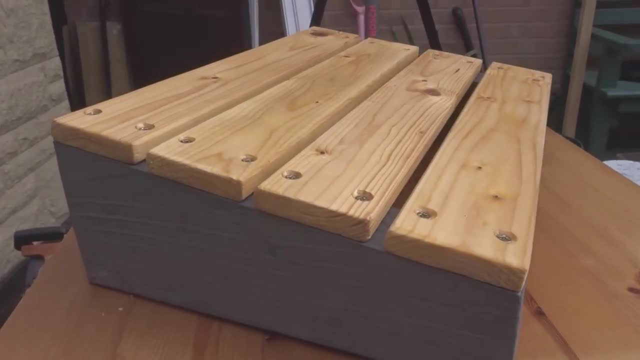 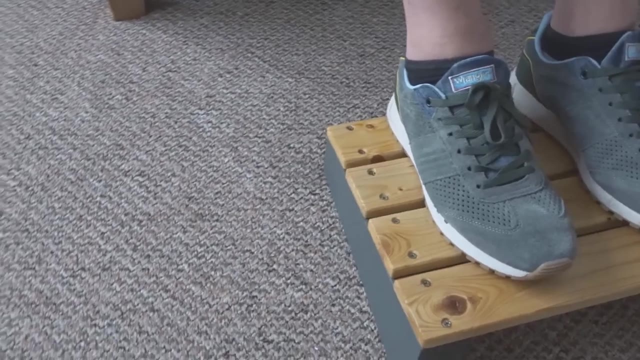 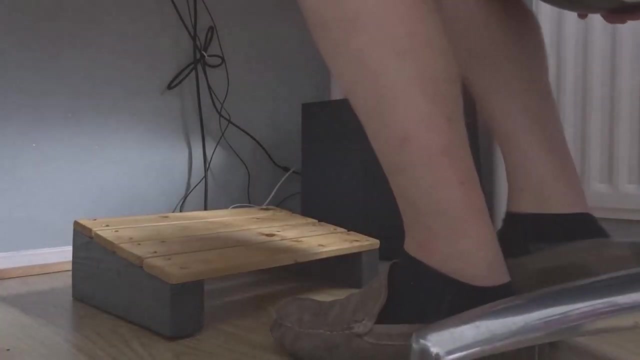 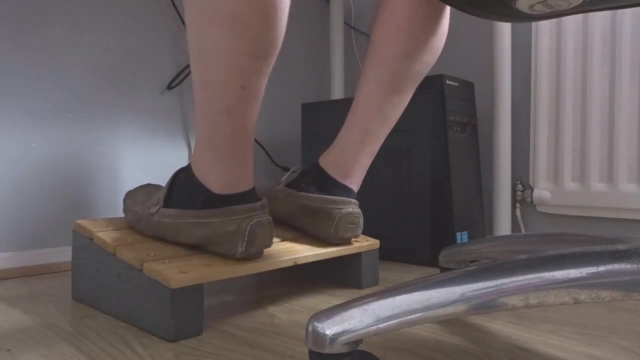 an old piece of two by four, and then a few old bed slats. These are great if you're working on a desk and you want to elevate your feet slightly, just for better blood circulation. So number two is a bottle opener. So all you need for this is any. 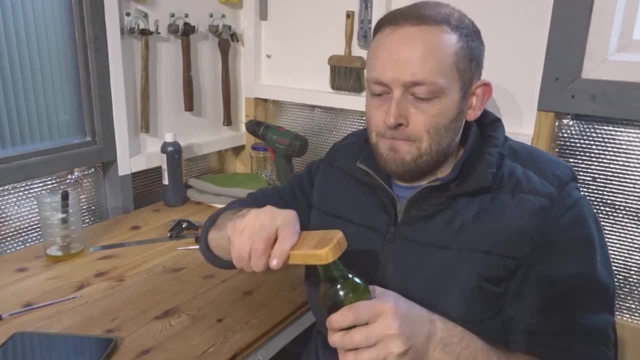 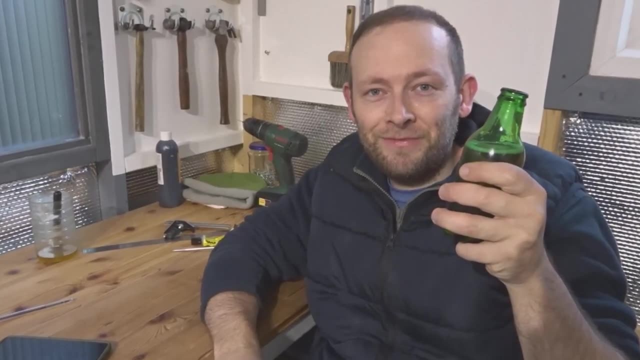 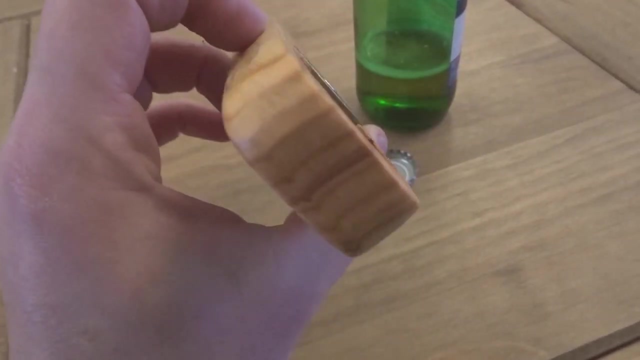 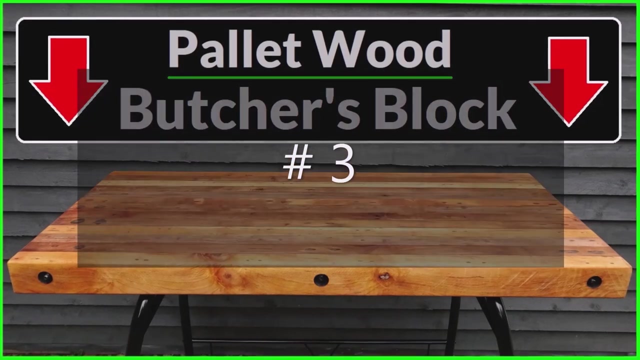 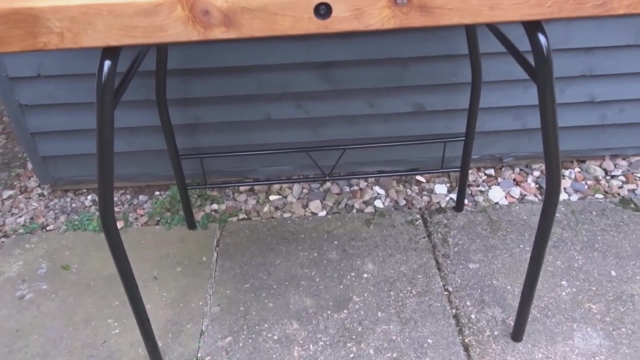 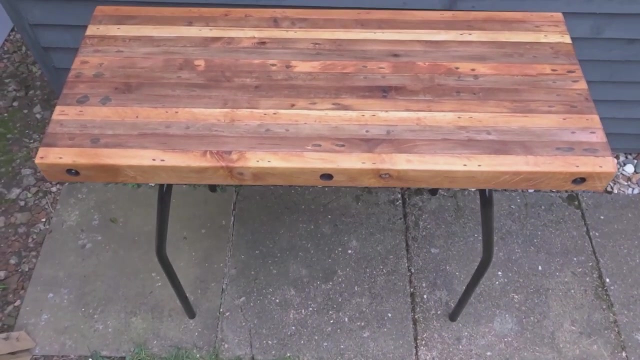 bit of scrap wood and an old coin, And these are great gifts. So number three is a butcher's block. I made mine for an office desk and for this I used the thick skid pieces of a pallet and I drilled some holes and put some bolts through and it makes a really chunky. 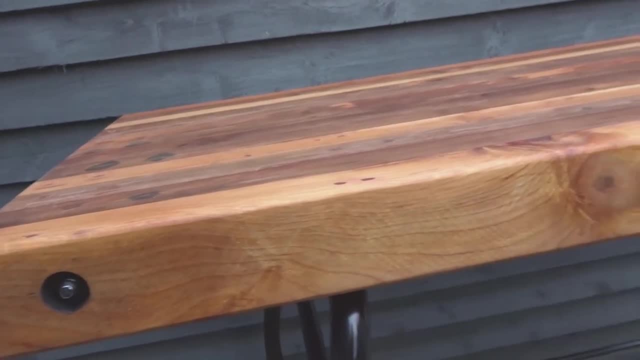 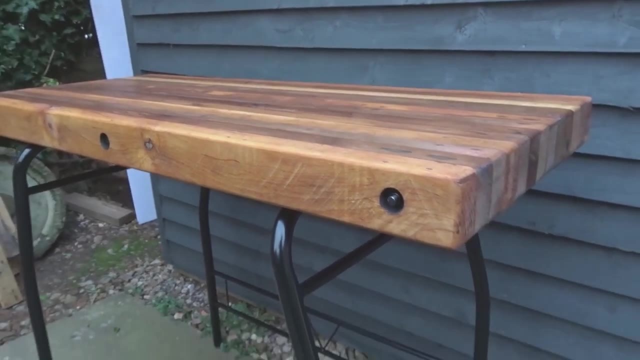 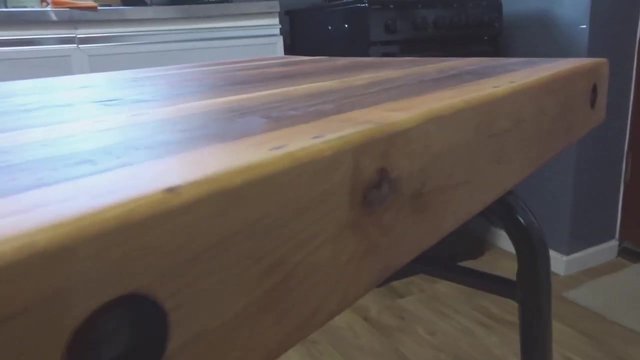 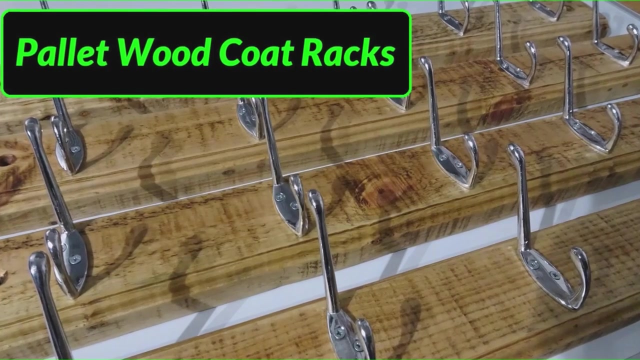 solid desktop which is made purely out of free wood. So number four is a pallet wood coat rack. Again, just a couple of pieces of a pallet, Just using the skid pieces from the pallets, and these make great gifts and these are good sellers. 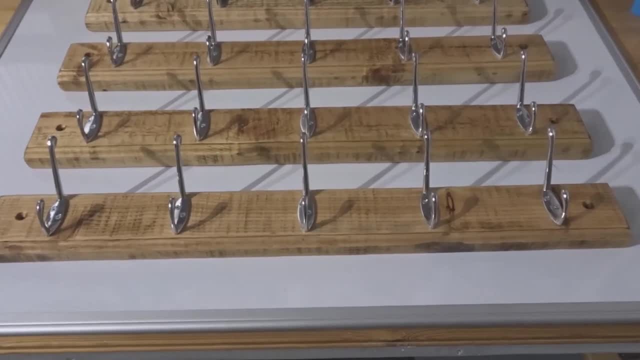 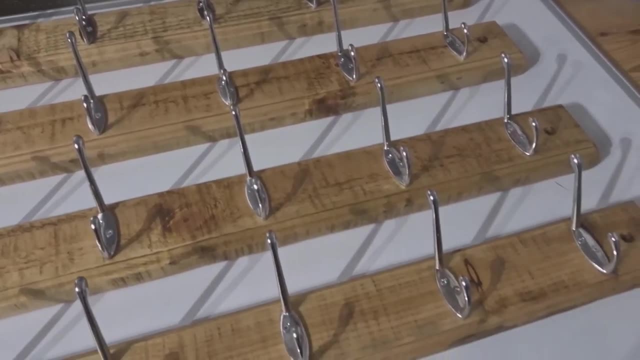 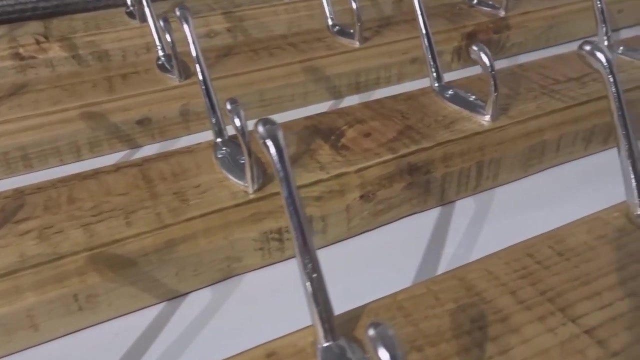 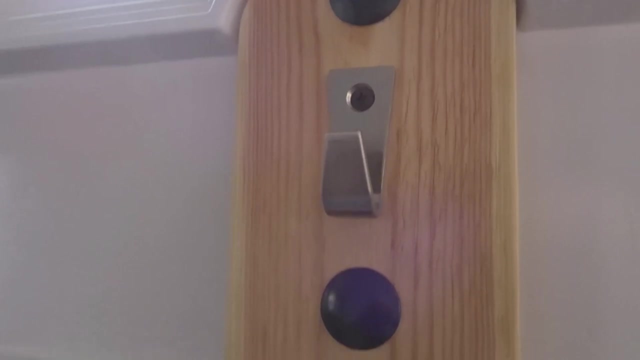 as well if you'd like to sell your woodwork. Very easy, very simple to make, And you can also make different variations of these. You can also make different versions of these. and you can also make different versions of these. You can also make variations like this key hook that I've put on the back of the door of my workshop. 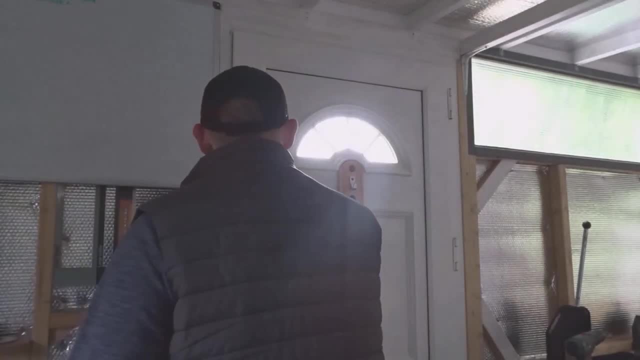 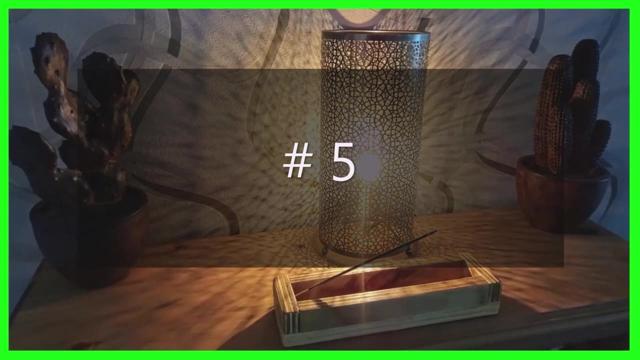 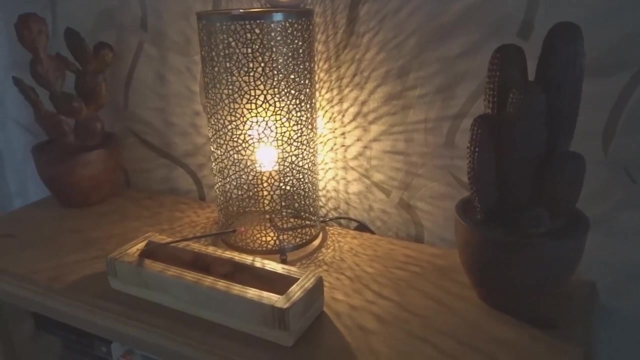 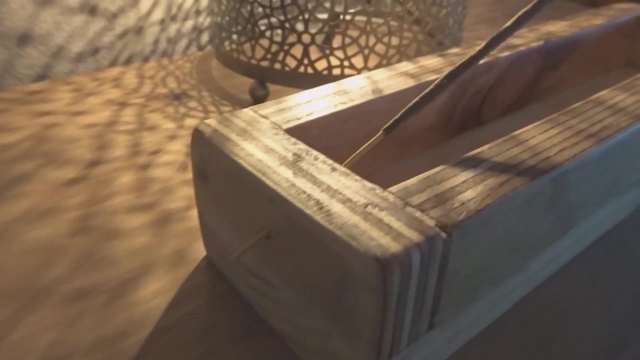 Number five is an incense burner. So I made this just out of a piece of scrap plywood. Great for burning incense, and the box just catches all the little dusty bits. Again a great gift or just great to use around your home. 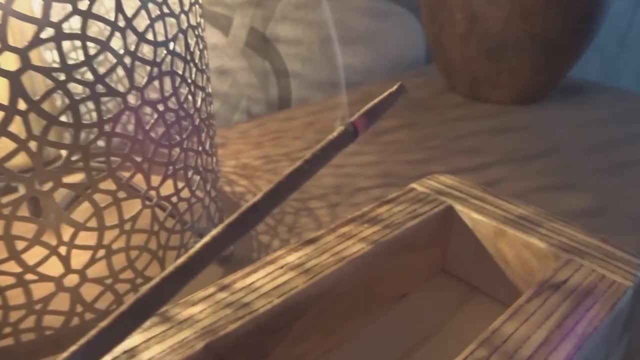 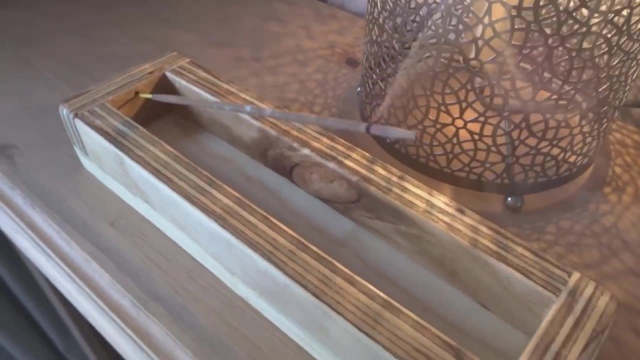 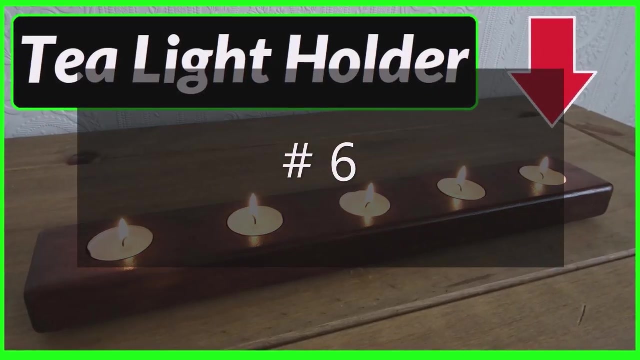 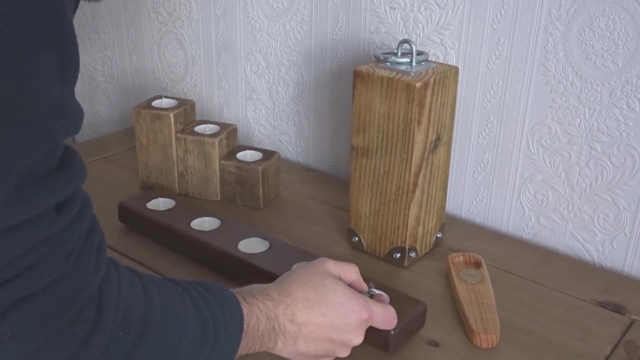 So number six is a tea light holder. You can make lots of different variations of these. Again, any old pieces of scrap wood will do. Number six is a tea light holder. You can make lots of different variations of these. Again, any old pieces of scrap wood will do. 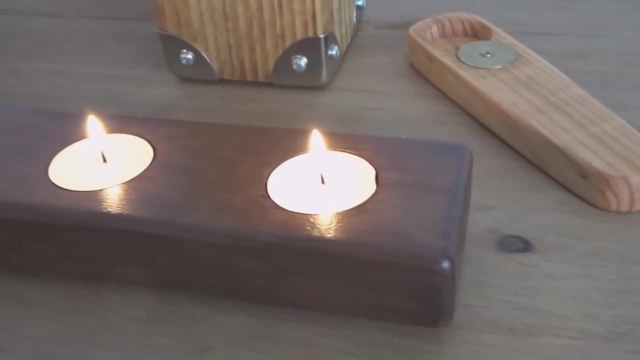 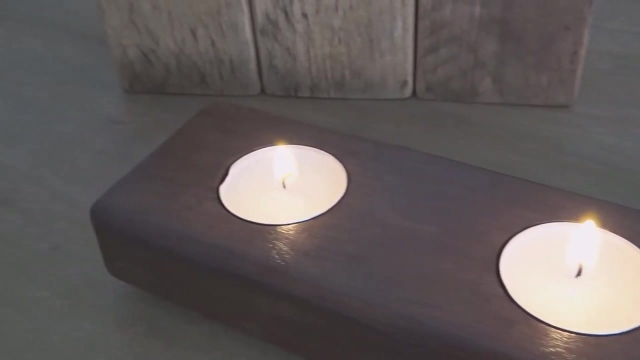 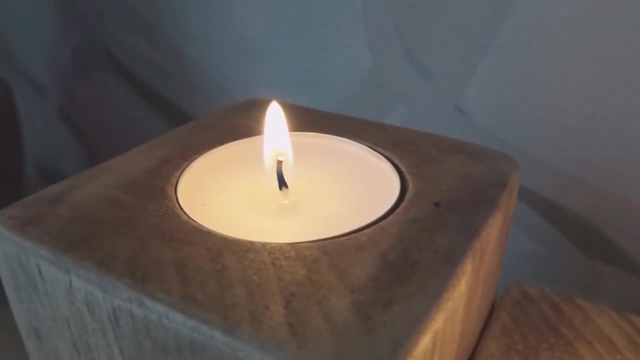 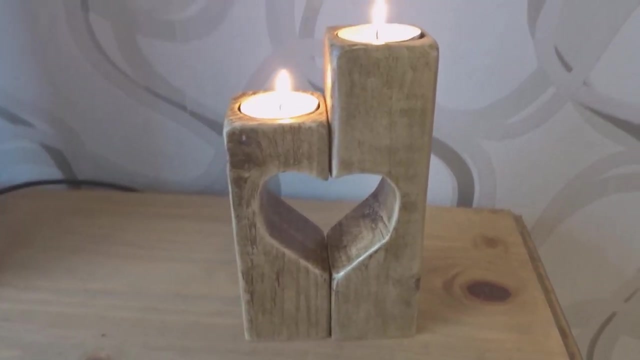 For that one I used again a pallet wood skid, Pretty much a piece of two by three or thereabouts, And for these these were just an old fence post that I found thrown out, And you can make different variations of these, like heart variations. 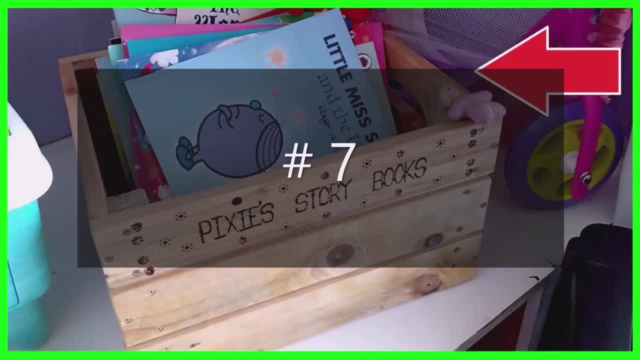 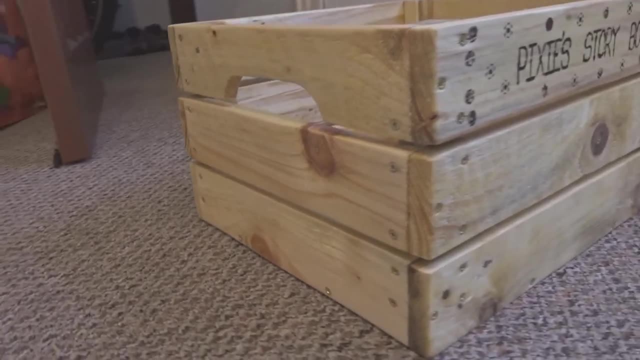 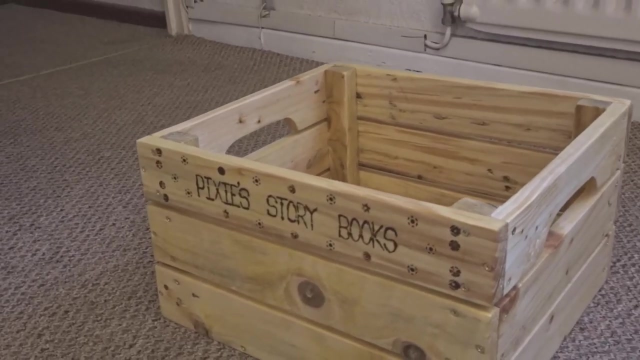 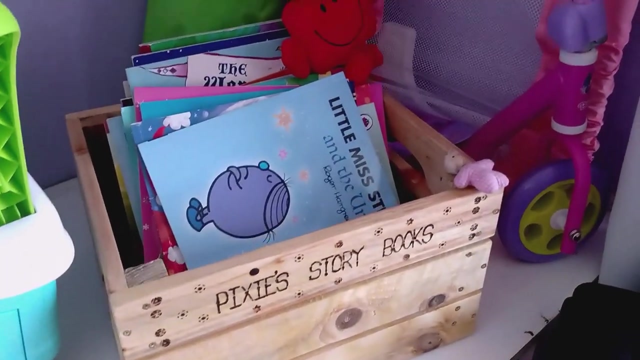 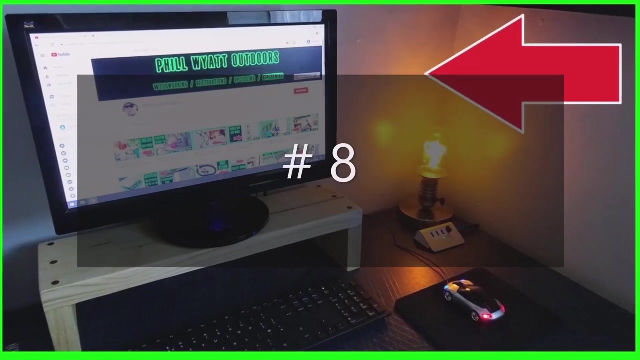 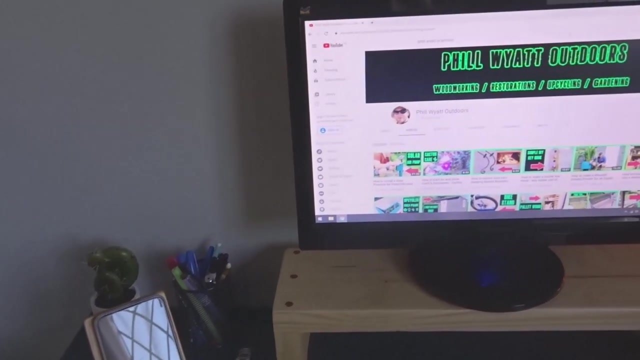 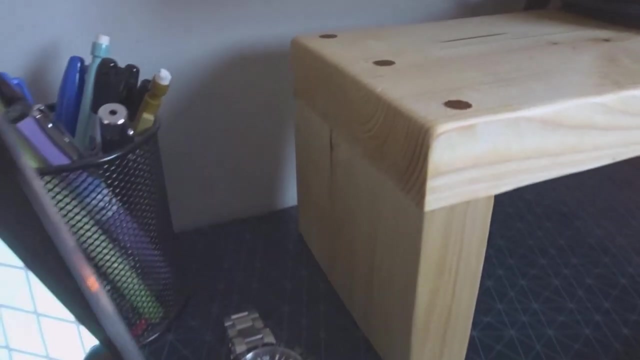 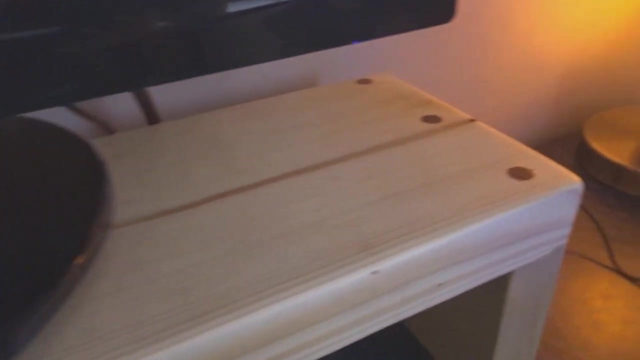 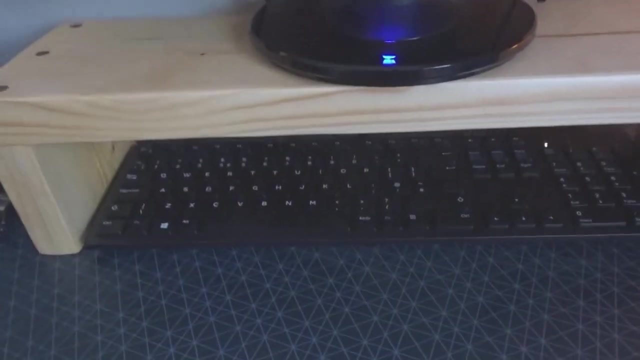 So number seven is a storage crate. So number 8 is a stand for your monitor, and this was just made out of one piece of wood that I found in a skip, and it's great to just elevate your monitor up so that your neck isn't bent downwards.